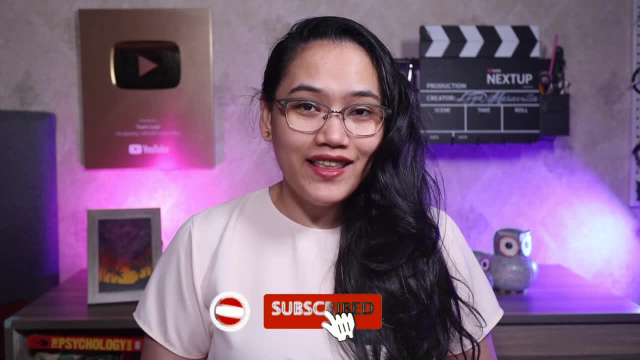 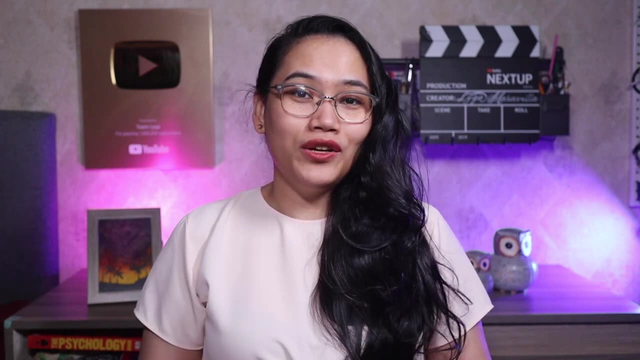 if you don't want to miss any of my new uploads, don't forget to hit subscribe and hit that bell icon. Now, like I said in the intro, we're going to talk about the different types of numbers and, of course, we're going to do a quiz at the end of this video. So if you're getting ready for an exam or 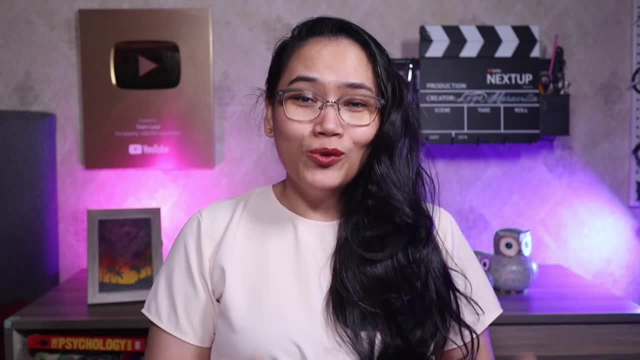 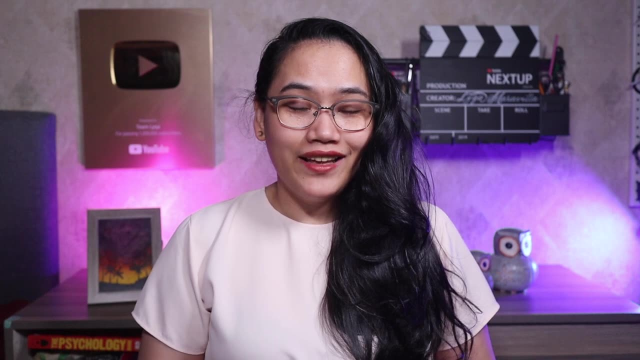 you want to have resources to help your children who are studying online and at home right now. stay tuned for that. And before we do that, just a quick little plug If you want to help support this channel and our cause to democratize education in the Philippines. one way that you can do that: 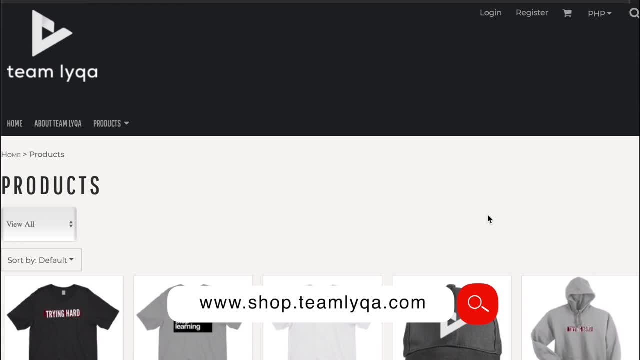 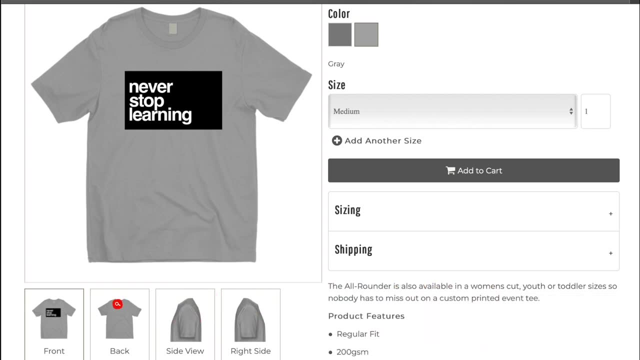 is through buying our merch at shopteamlaikacom. You can go and check that out for our shirts, hoodies, caps and other things I designed for this team. Thank you so much for buying our merch, And if you can't afford to do that right now, that's perfectly fine. Again, this is just us. 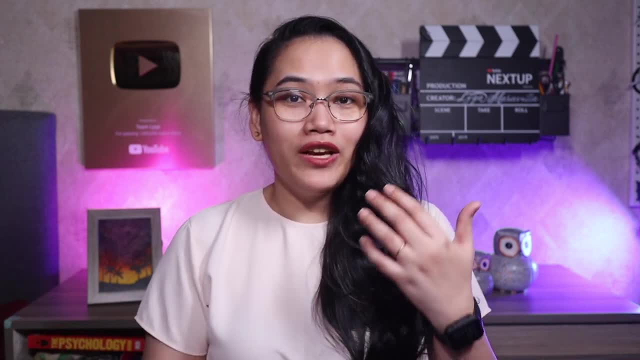 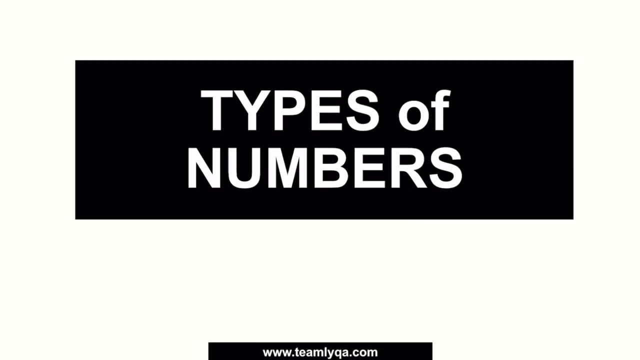 helping the team to make sure that we can keep creating free content for all of you. Now that we have that out of the way, I'm going to switch over to my tablet. I'll see you in a bit. Okay, so this is our discussion on the different types of numbers. We're going to try our best to be as 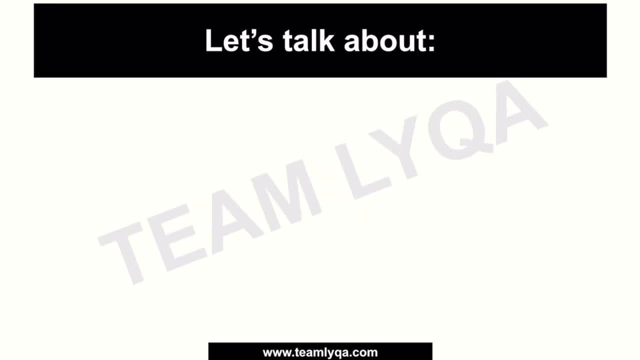 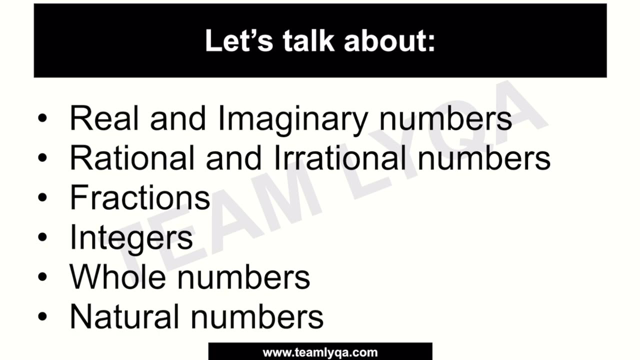 simple to as possible. We're going to start off by listing yung mga pag-uusapan natin. ngayon. We're going to talk about real and imaginary numbers, rational and irrational numbers, fractions, integers, whole numbers and natural numbers. Okay, now isa-isahin natin ha per level. 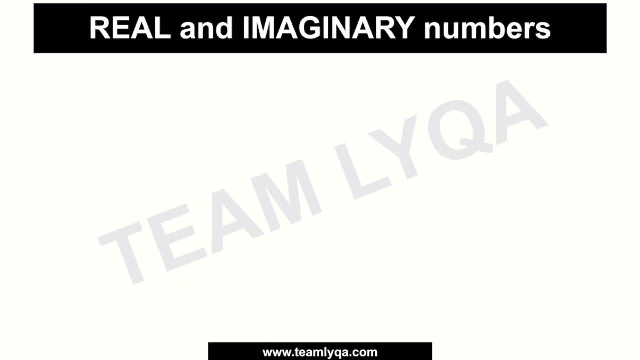 The first thing we're going to talk about are real and imaginary numbers, Ibig sabihin ito: itong dalawang bagay na ito ay magkaiba Yung una would be. yung bagay na ito ay magkaiba Yung una would be. 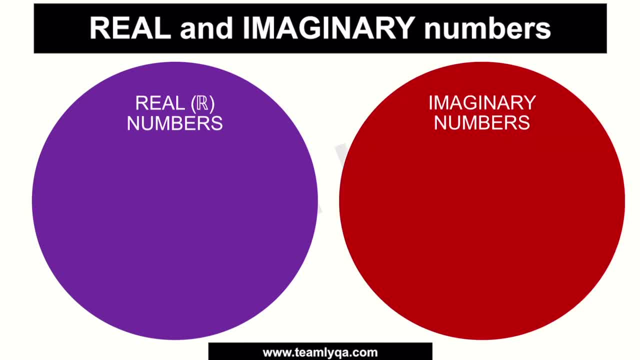 yung real numbers and yung sa kabila naman ay imaginary numbers. Now again ha nakikita natin- I'm trying to use the Venn diagram here para mas visual sa inyo- Sila ay magkahihwalay Walang. 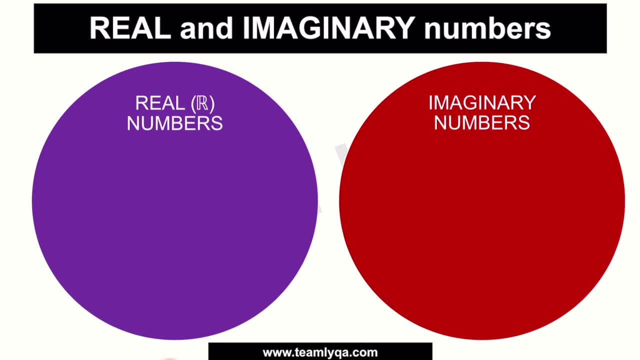 number na real na imaginary pa Okay, So wala rin imaginary na real pa Magkaiba sila. Each number can only be one of these two. Now ano yung definition nila? When you talk about real numbers, siya ay nabubuo ng mga rational and irrational numbers. 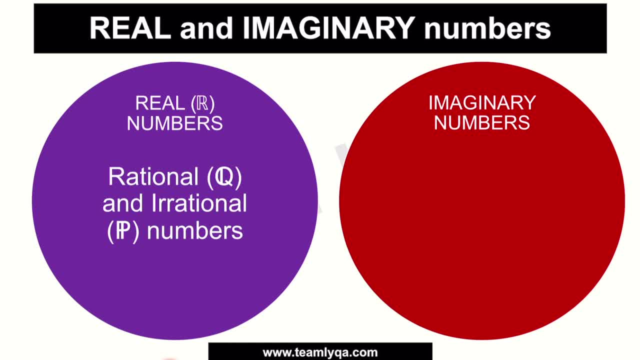 In some definitions ang sinasabi ito ay ang union of the set of rational and irrational numbers. Now we're going to talk about those in a bit. Dito muna tayo mag-focus sa imaginary numbers. Ang definition ng imaginary number ay: 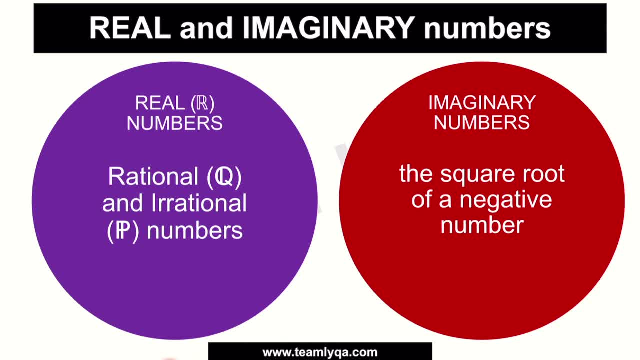 ito ay square root of a negative number. Kadalasan natin ginagamit ito with the symbol na I And ang I na yan ay equal to the square root of negative 1.. Now yung conversation on imaginary numbers and complex numbers. 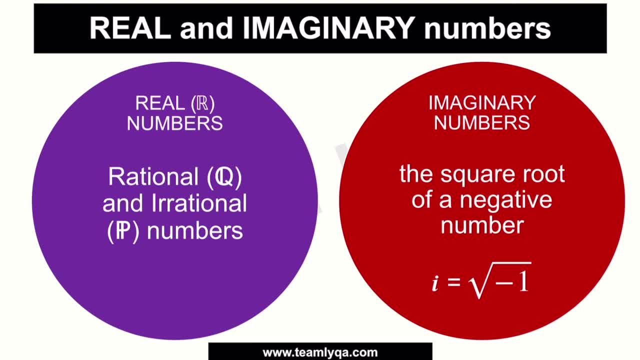 that is another story for another time. Most naman ay kinukover yan sa pagdating nila sa advanced math. Pero ang importante, mag-focus tayo on the set of real numbers, kasi ito yung usually lumalabas sa mga exams ninyo. 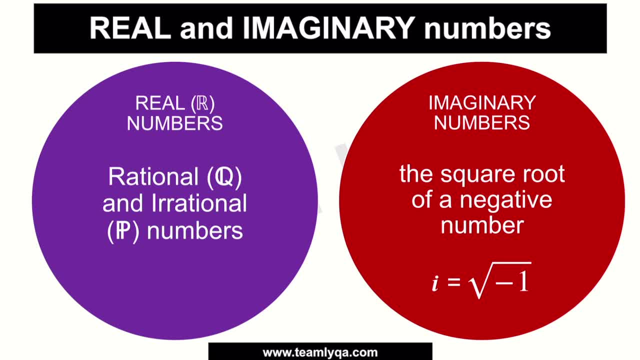 And ako personally yung nag-upcut ako ito. yung isa sa mga problems na natatandaan ko ay merong ganitong klaseng tanong. Okay, Now, if ito yung lahat, lahat ng real numbers. 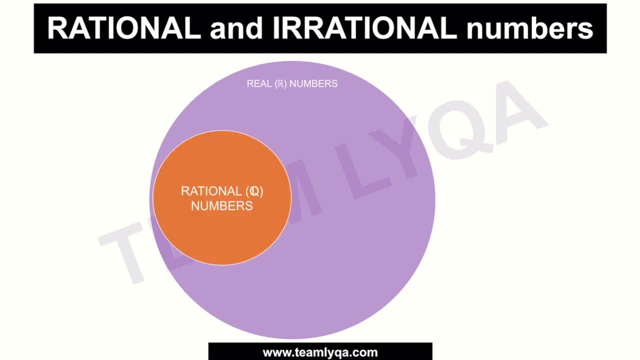 again, this is just for visual purposes. masasabi natin na ang rational numbers at irrational numbers ay real numbers, silang lahat. Okay, Anong ibig sabihin ito? Ito? ha again, kasi dahil lang kulang tayo sa illustration. 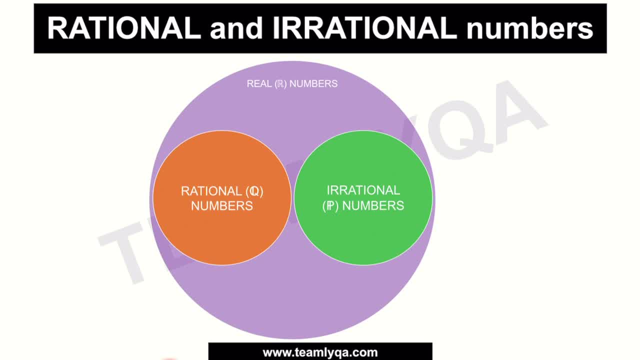 itong numbers na ito, kumbaga nakahati ang real numbers sa rational numbers at irrational numbers, and wala ng iba. Okay, Alam ko medyo may empty space tayo dyan, pero isipin ninyo na walang laman ito. 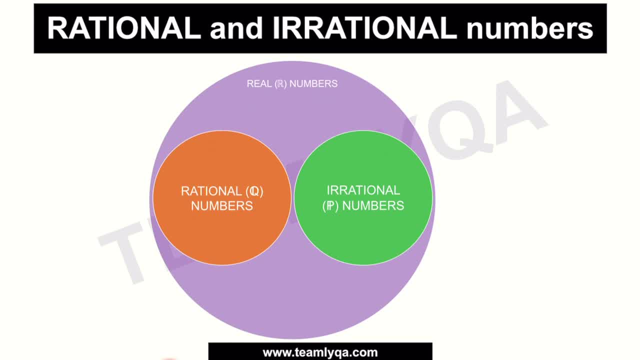 Okay, So non-real numbers can either be rational or irrational. Hindi rin pwede na rational na siya, irrational pa siya. Okay, Hindi pwede yun. But you would notice na kung ang number ay rational number, automatic siya ay real number. 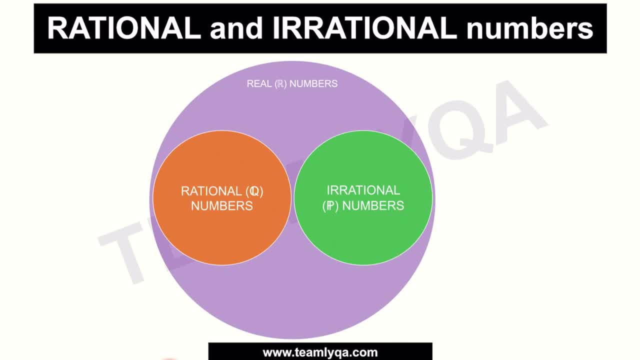 At kung irrational number siya, siya ay automatic na real number din. Now tinan natin yung definition. Rational numbers can be expressed as the ratio of two integers, For example P over Q, where Q is not equal to zero. 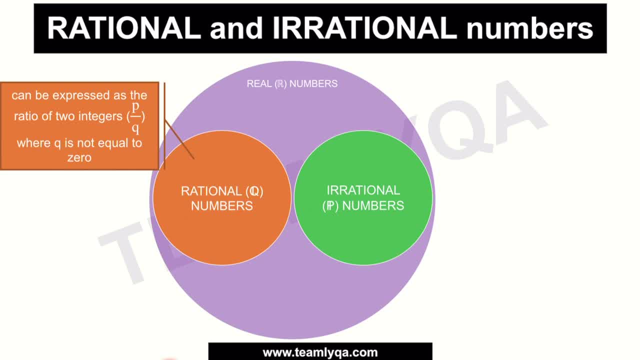 Now, ano lang ibig sabihin ito? Ang mga rational number. pwede mo siya isulat as a fraction, tapos yung kanyang denominator. yung number sa ilalim ay hindi zero. Now, kung titinan natin yung definition ng irrational numbers, 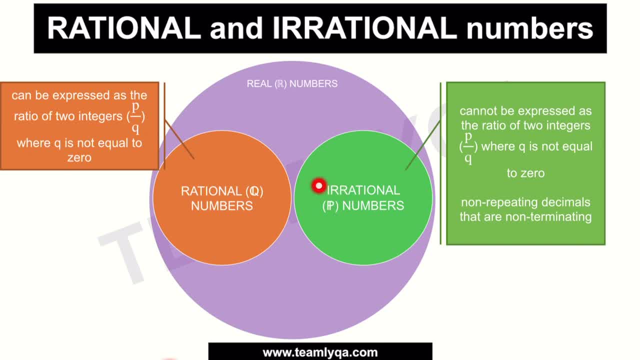 kabaliktaran siya no, Kasi nakikita natin di ba pag may prefix tayo na IR irreplaceable, yung mga ganon di ba. irreparable ibig sabihin hindi siya ganon. 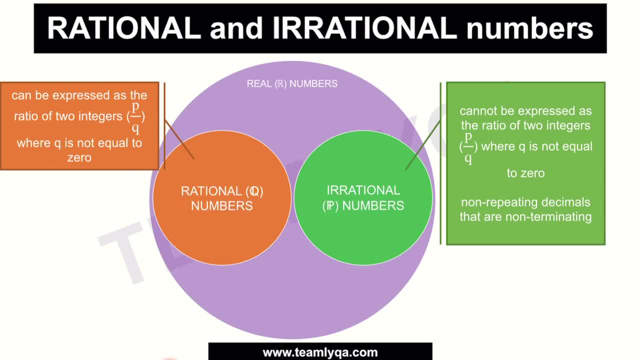 So kung hindi siya rational, irrational siya, Which also means na ang definition niya is those that cannot be expressed as the ratio of two integers. Ibig sabihin, nun, hindi siya maisusulat as P over Q. 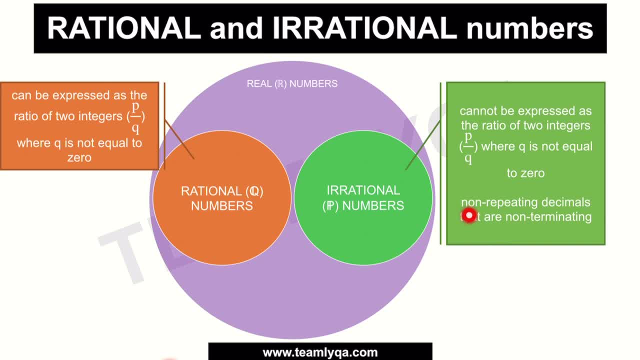 Clue natin yung fact na these are also non-repeating decimals, that are non-terminating. Now, ano ibig sabihin? nun, We will see in a bit. no, Kasi. I'll give you a few examples. 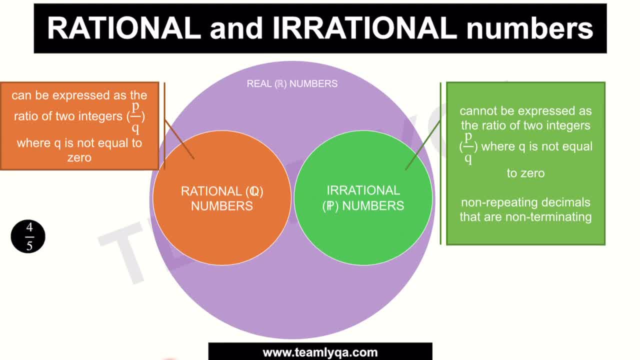 Now here's the next task. Kung meron tayong 4 over 5, is it a rational number or an irrational number? Now again sabi natin kailangan pwede siya isulat as P over Q, at hindi zero yung Q. 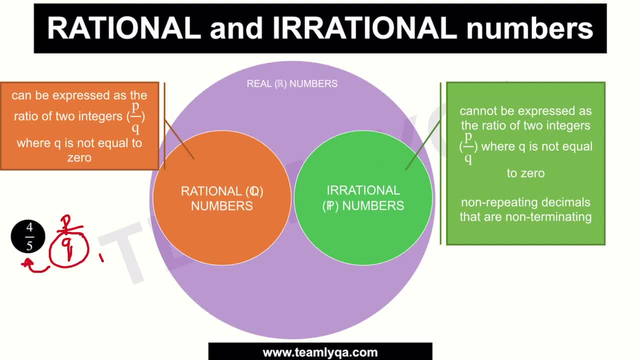 Now yung 5, hindi naman siya zero. So check tayo, dyan Yung 4 ba ay integer Yes. So ibig sabihin nun ang 4 over 5 is a rational number. 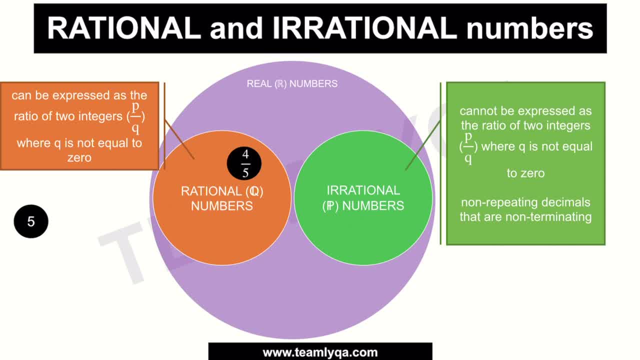 Now, if you have something like 5, naman ang 5 ba rational or irrational. Now sabi natin it should be expressed no, Or pwede siya i-express as a fraction, like this, kung rational number siya: 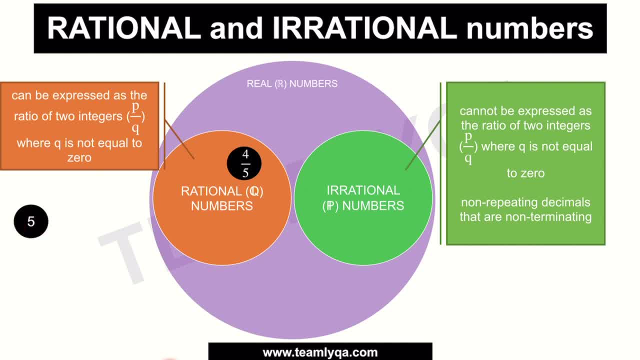 Now I know, wala tong hindi siya naka-fraction form. no, Pero ang 5 kasi ay pareho lang sa 5 over 1, no, So ibig sabihin pareho lang yan, equal lang yan. 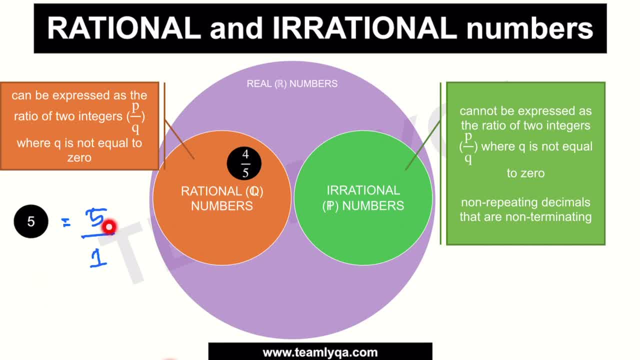 It can be written as 5 over 1.. And because ang 5 is an integer, ang 1 is an integer at hindi siya zero. ibig sabihin, ang 5 is also a rational number. Now let's look at negative 3.. 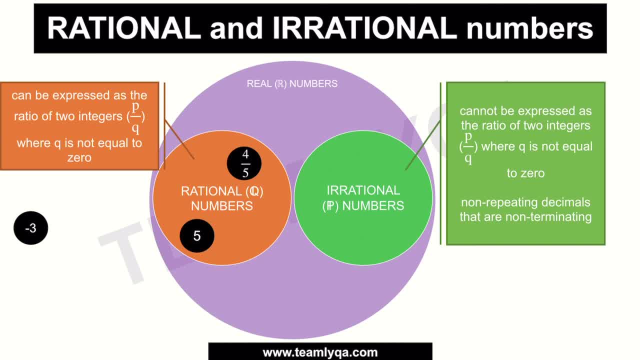 Ang negative 3 ba ay rational or irrational. Sulat din natin siya as a fraction. Ito ay negative 3 over 1.. Now, is 3 or is negative 3 an integer? Yes, Is 1 an integer, at hindi siya zero. 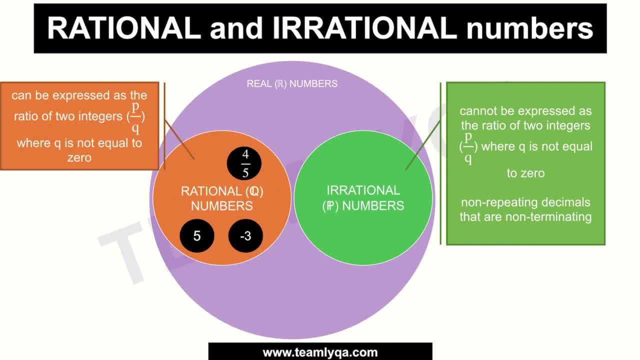 Yes, So ibig sabihin rational number din siya. Paano naman ang pi? Now, ano ba ang pi? Ito yung ginagamit natin diba sa formula ng circles. And if you haven't seen, 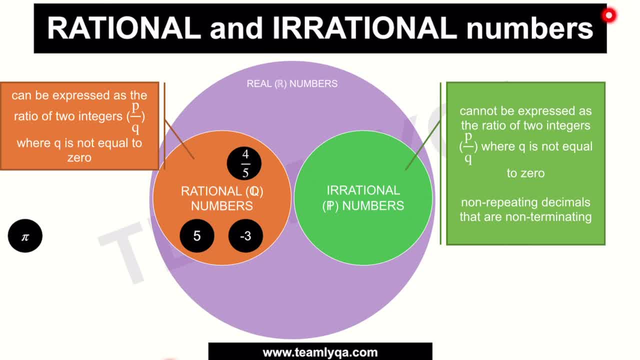 yung video natin sa area circumference ng circles. click right here na lang sa i-button if you're watching on YouTube, ha, Or sa description box sa baba. Now, ang pi is actually a non-repeating and non-terminating decimal. no. 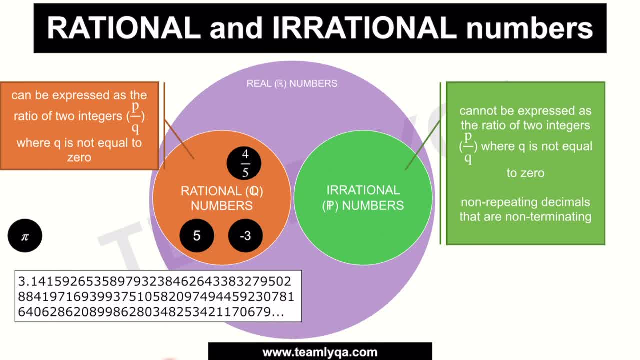 Meron siyang mahabang-mahabang list ng mga numbers na yan And a quick little trivia nga dun sa memory Olympics. isa sa mga categories nun ay ang pag-memorize ng mga digits ng pi. Paramihan ang mga tao. 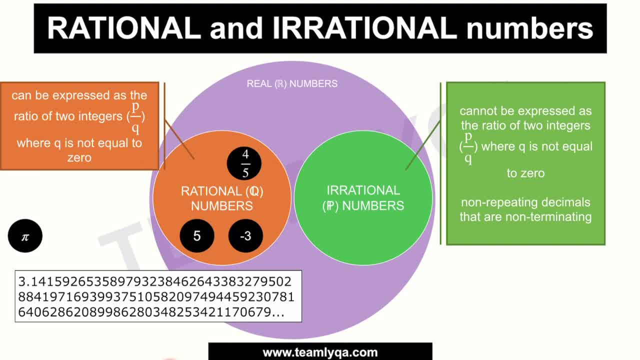 Nang hanggang kailan nila ma-memorize yung dami ng mga digits na yan sa dulo. So dahil check siya, kasi hindi siya repeating, ibig sabihin hindi nauulit yung dalawang digit lang, isang digit lang o ilang digit lamang. 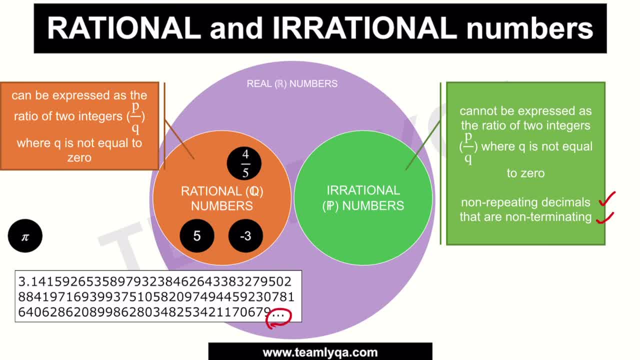 At siya ay non-terminating kasi hindi siya natatapos. no, Then ibig sabihin nun ang pi dito siya mapupunta, siya ay irrational number. Now, if you have something like 0.6 na may bar sa ibabaw. 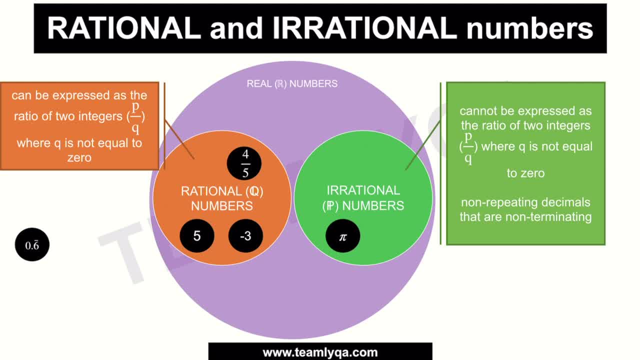 ibig sabihin ito ay repeating decimal, Which means di ba hindi siya non-repeating. di ba Kaya. alam na natin agad. rational number siya. Now, if you want to check by converting it into a fraction: 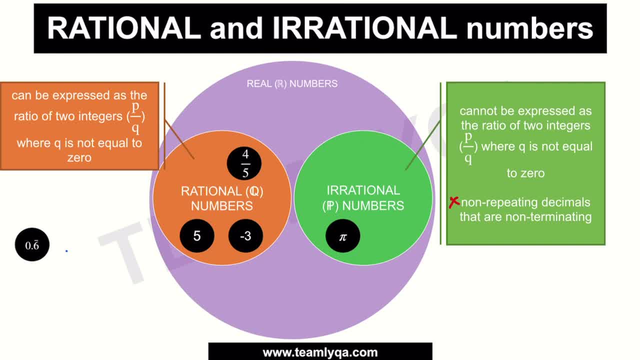 you will also know na ang 0.6 na repeating, or kung isusulat natin yan, ay 0.6 na paulit-ulit. di ba Naulit lang yung 6, paulit-ulit yan. 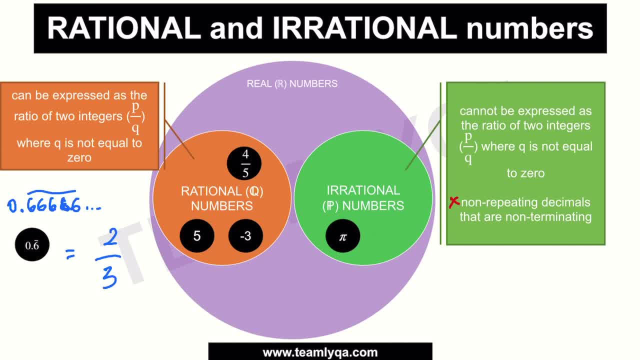 ay equal, yan sa 2 over 3.. Which ang 2 is also an integer 3, integer na hindi 0.. So ibig sabihin, nun siya ay rational number. Now, kung naguluhan kayo kung paano ko nalaman na 2 over 3 yung 0.6 bar. 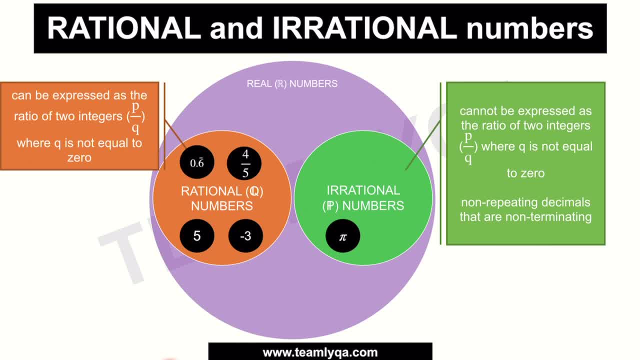 na yan na repeating decimal. meron tayong video din on how to convert repeating decimals into fraction In sa kanyang fraction form. ililingko na lang din dito sa taas sa i-button. Okay, Pwede niyong panoorin yun. 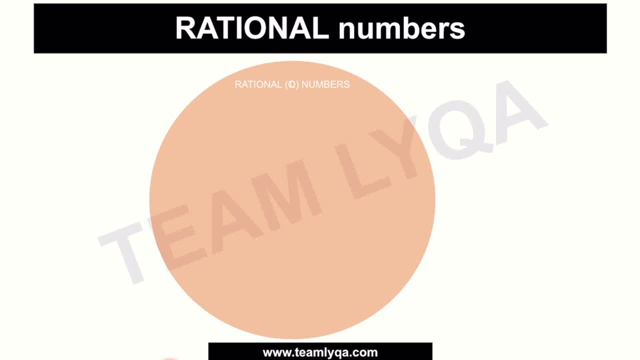 Now, Now alam na natin kung ano yung mga rational numbers, And rational numbers can include yung fractions and integers Na hindi ko na point out. kanina, may mga symbols na ganito: no Yung, yun ay kumakatawan sa integers. 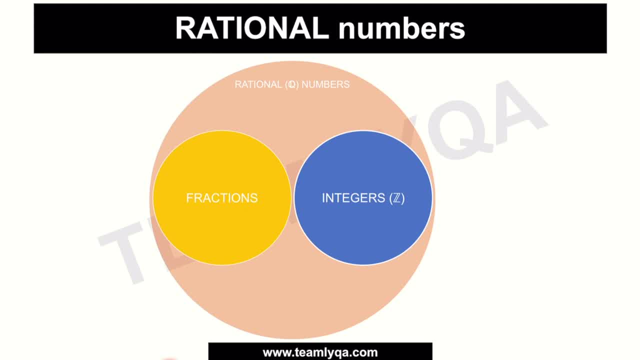 ito namang Q ay kumakatawan sa rational numbers at iba pa. no, Now isa-isahin ulit natin yung natira dun sa listahan natin ng rational numbers, Ang 4 over 5, dahil meron siyang numerator at denominator ay fraction. 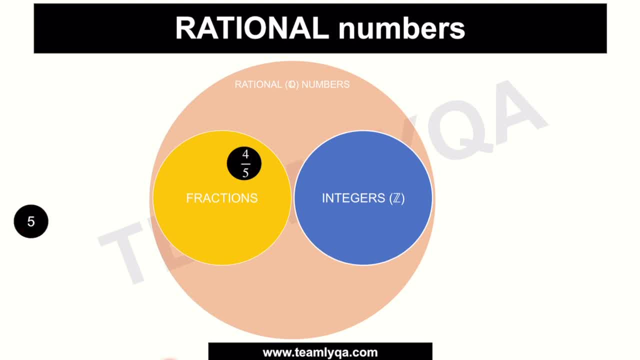 Ang 5, dahil meron siyang denominator at denominator ay fraction. Ang 5, dahil meron siyang numerator at denominator ay fraction, Dahil siya ay buo no Ay integer Ang negative 3, dahil buo rin siya kahit siya ay negative no. 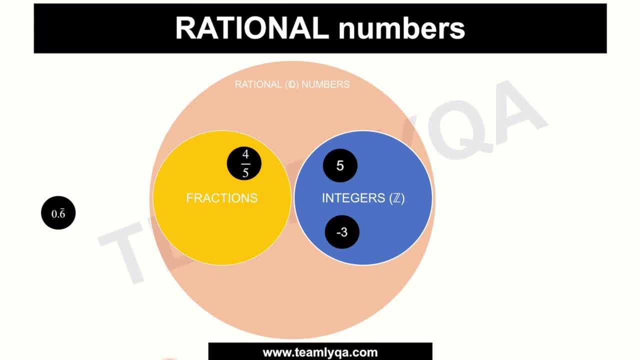 Kasi meron tayong negative integers, siya ay negative. Ang 0.6 na repeating number, again no. Na equal din siya, or equivalent siya sa 2 over 3, yan ay fraction, Kaya nga again no. 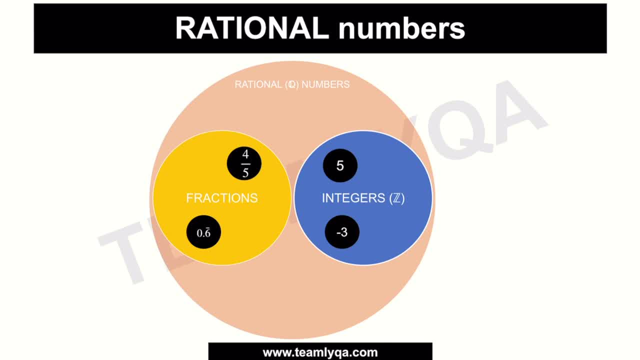 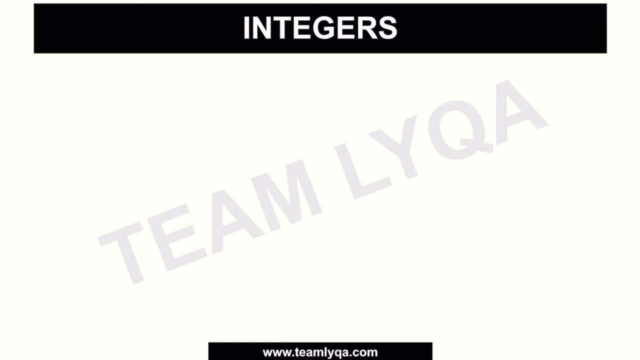 Very important for us din to know how to convert decimals into fractions, fractions into decimals, And again, we have an entire playlist na dedicated to that. Now, dito naman tayo sa integers Kung baga, let's take a closer look. no. 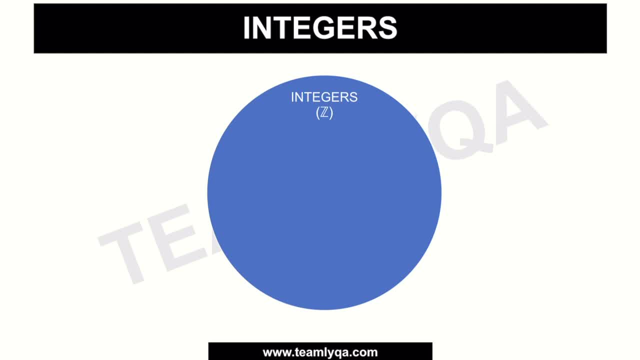 Kung lahat ng mga integers ay nandyan. ang mga integers ay ang whole numbers kasama ang 0, pati ang negative nitong mga whole numbers na ito, meron naman tayong tinatawag na whole numbers. 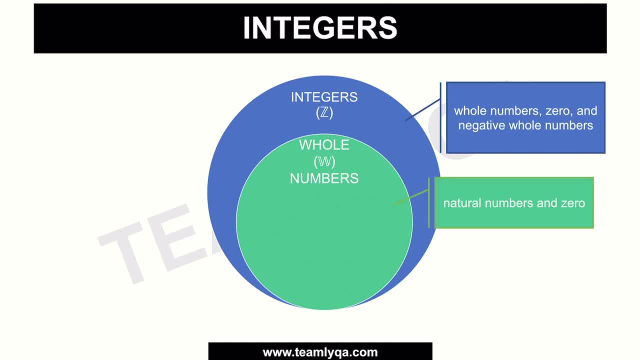 which are yung mga natural numbers and 0,. at yung natural numbers naman are our counting numbers. Now, kung medyo naguluhan, kayo doon na alin ang alin dito. let me give you a few examples. 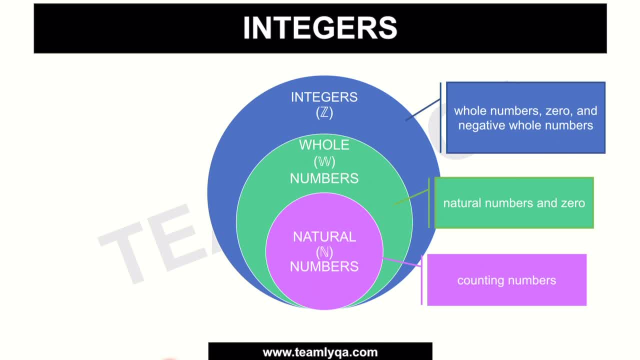 Pagdating sa natural numbers, ito rin yung tinatawag nating counting numbers. kadalasan tayo nagsisimula sa 1.. So you have 1,, 2,, 3,, 4,, 5,. 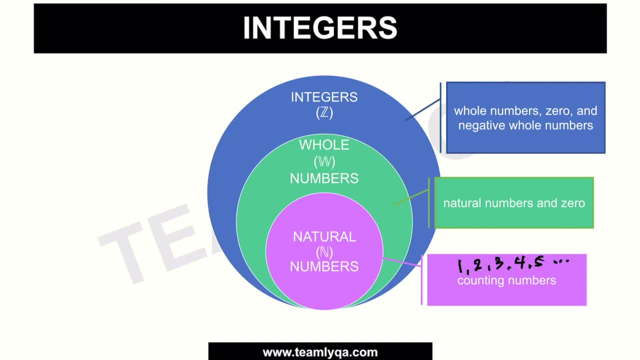 at yung mga susunod pa na buong numbers nakasunod niyan Ang natural numbers. naman, pag dinagdag mo na ang 0, yan na ang tinatawag nating whole numbers. The idea is kasi hindi naman tayo nagsisimula sa 0 kapag tayo ay nagbibilang. 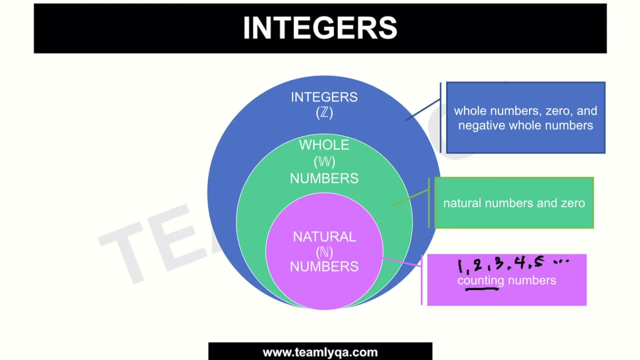 kaya yun yung counting numbers. This time kasama na siya pagdating sa whole number, Kasi whole number din ang 0.. So now you have 0,, 1,, 2,, 3,, 4,, 5,. 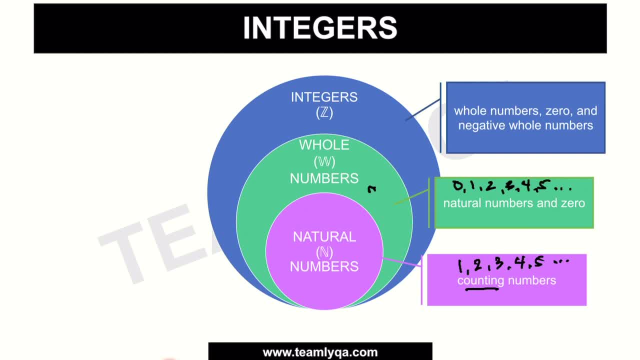 at ang mga susunod pa sa kanya. Now, pagdating sa integers, mas malaki na yung ating circle, Kasama na dyan yung counting numbers, yung 0, pati yung negative ng mga whole numbers natin. 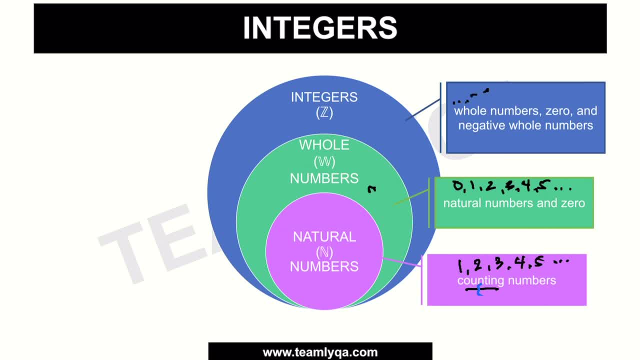 Yan. infinity din yan. no, Kasi, tuloy-tuloy yan. Then you have your negative 3, negative 2, negative 1, zero, and then 1,, 2, 3, sunod-sunod na yan. 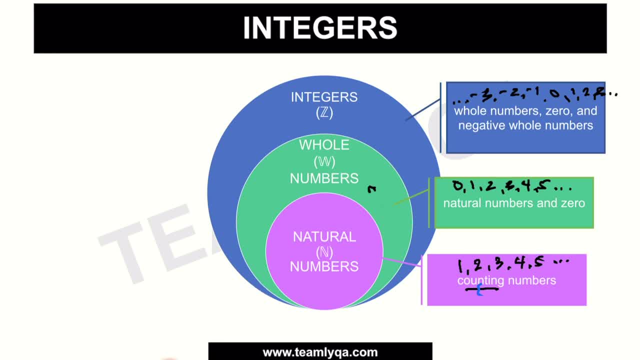 Okay Now, bakit ganito yung pagkakasulat ko sa kanila? I'm hoping na makatulong to sa inyo to remember things. Bakit? Kasi lahat ng natural numbers ay whole numbers, Kung baga dun sa Venn diagram na logic lesson natin. 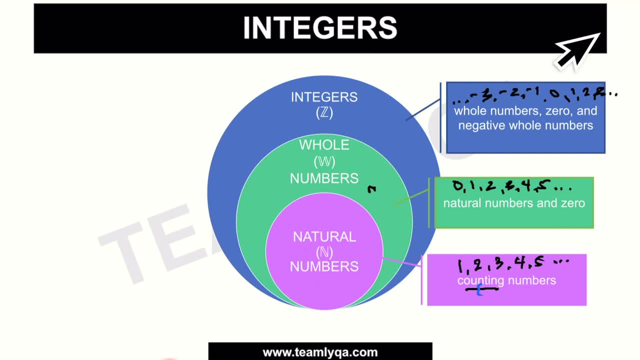 it's all. I-link ko din dito yung lesson na yun, just in case you need a little bit of help. But the idea is again, all natural numbers are whole numbers. Now, ano pinagkaiba niya. 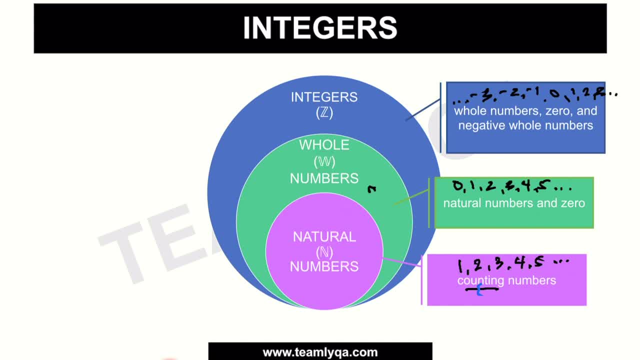 Pagdating sa whole numbers, kasama na ang zero, Para masudaring tandaan, isipin ninyo yung zero nandito sa whole, ng whole. Okay, So parang ibig sabihin may zero, siyang kadugtong. 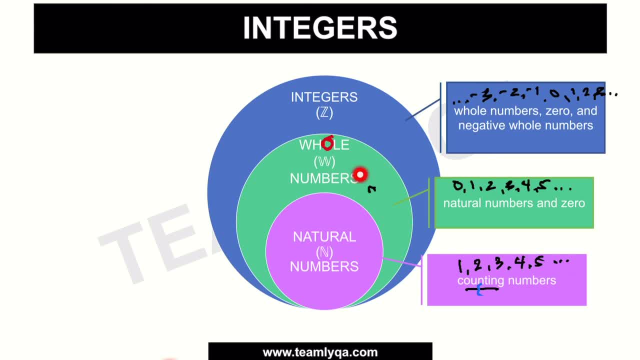 So all natural numbers are whole numbers. All whole numbers naman are integers. Okay, Pero hindi lahat ng integer ay whole number, at hindi lahat ng whole number ay natural number. Okay, Parang ganito yan. Okay, Natural numbers, ang tuta. 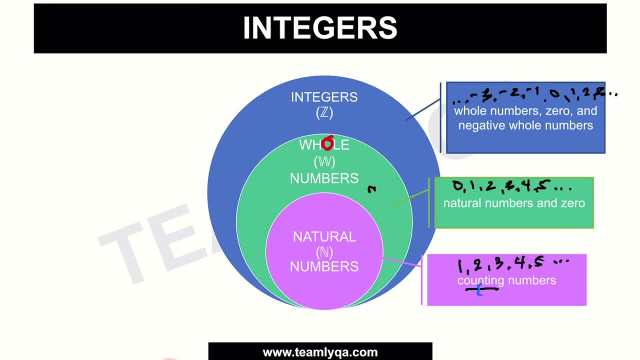 whole numbers. ang aso integers, ang canines, Ang mga tuta ay aso rin, Tama Kasi mga batang aso sila. Ang mga aso ay canines, Ang mga tuta ay canines din, Pero hindi lahat ng canines ay aso. 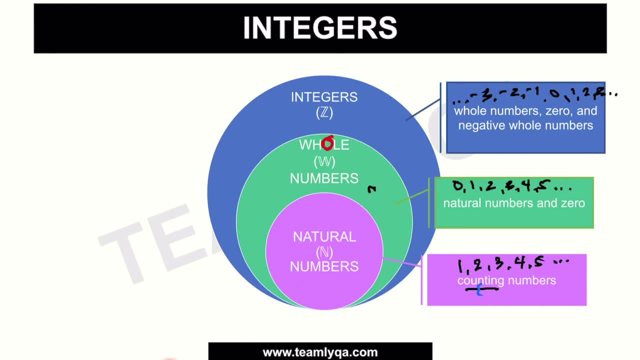 dahil may mga wolves, no Marami pang ibang klaseng mga canines, At ang mga aso ay. hindi naman lahat ay tuta, kasi may mga full grown ng aso. Okay, So just something. 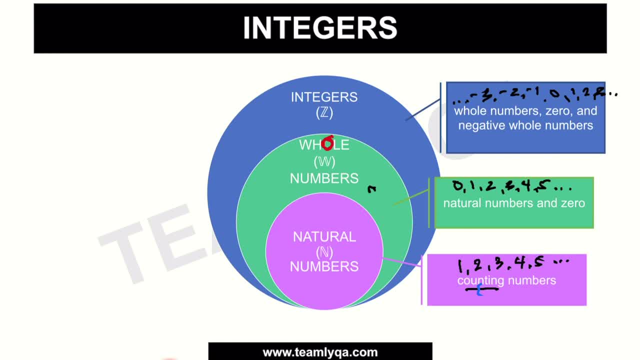 something to visualize pagdating sa conversation na ito. Now, if you look at yung ating mga numbers, kanina, you have five. Now ang five, saan ko siya ilalagay? Ang five ba ay integer. 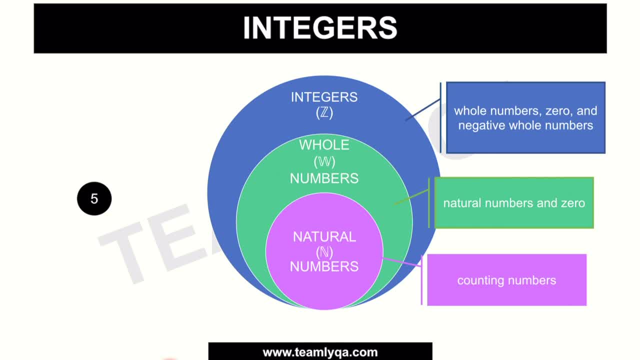 Dahil siya ay whole number positive, siya integer siya. so check dyan: Whole number ba siya Yes, Natural number ba siya Yes. So ang ilalagay ko would be: ang five ay natural number. 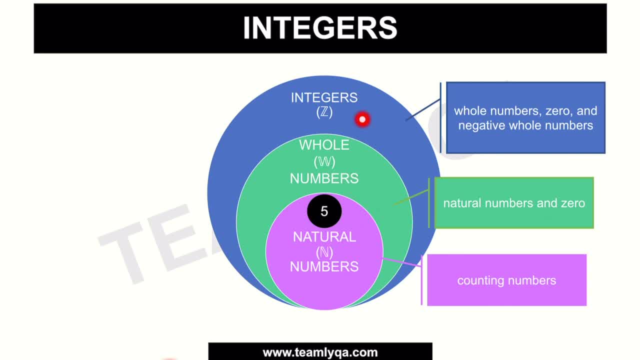 Natural number, whole number at integer. Kasi automatic again, lahat ng natural ay whole, din lahat ng whole ay integer. So check siya sa lahat ng tatlong bilog. Now, if you take a number like negative, three naman. 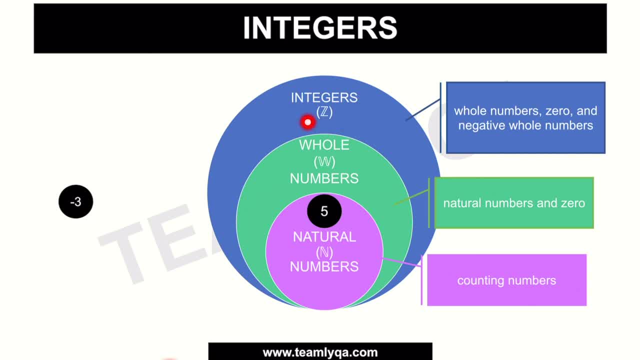 ang negative three ay integer Right, Kasi kasama doon ang negative whole numbers, Pero hindi na siya whole number, dahil hindi kasama ang mga negative dito. Hindi din siya counting number, kasi ang counting number kumaga lahat sila nandun sa right side. 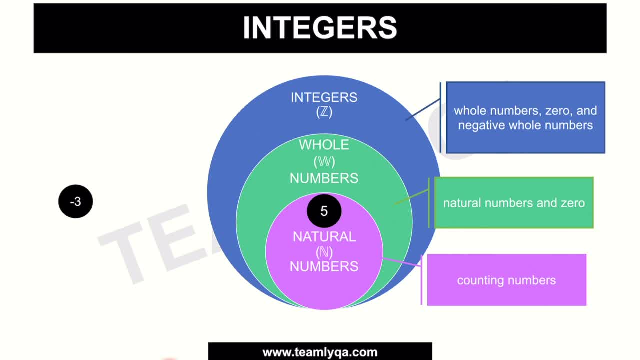 Ibig sabihin mga positive numbers ito. So ibig sabihin nun, ang negative three ay integer, pero hindi siya whole number at hindi din siya natural number. If we have something like zero, naman no. 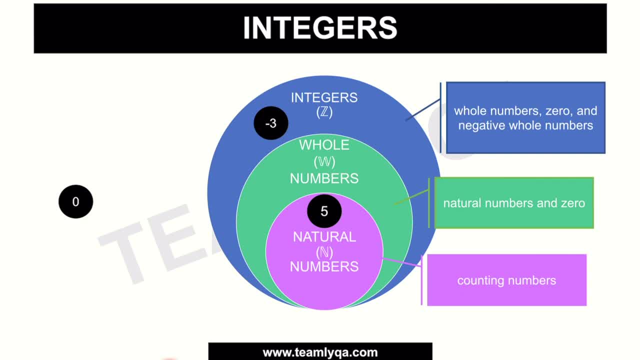 Ang zero ay integer, yes, kasi kasama siya doon Ang zero. ay whole number, kasi kasama doon ang zero, pero hindi siya counting number. So kung ilalagay ko siya dito, ilalagay ko siya dyan. 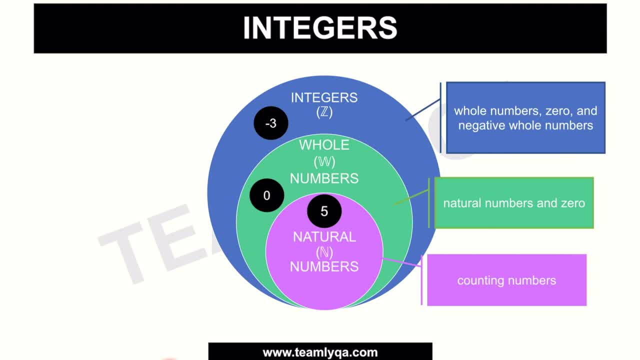 Okay, Now again, it's important for us to know which is which May mga certain rules na nag-a-apply sa bawat isa sa kanila. At syempre importante for us to know, lalo na kung nagsasolve tayo ng mga equations. 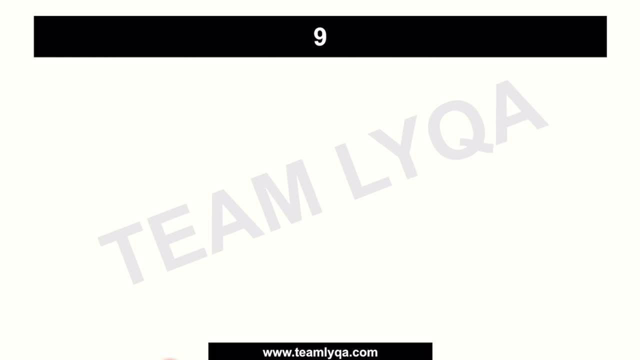 Now, paano natin ito, mamamaster, Let me give you another visual representation. Kung meron akong number na nine at gusto ko ma-figure out kung anong type ng number siya, this is a lot like yung exercise natin pagdating sa types of nouns. 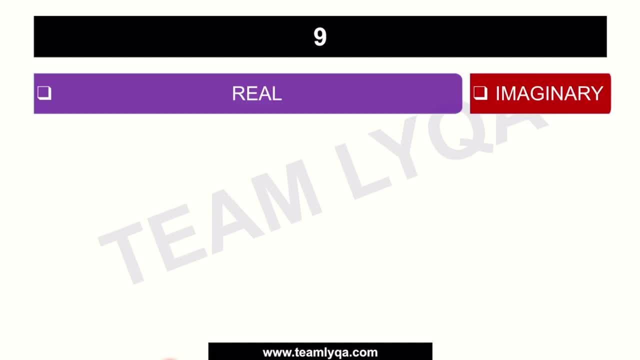 First level. unang tanong: is it real or imaginary? Now, dahil ang nine ay real number, hindi siya imaginary, hindi naman siya square root of a negative integer. siya ay real, So check natin siya dito. 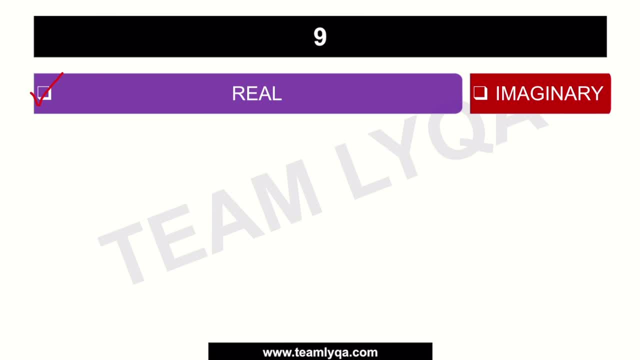 Now, dahil siya ay real number, bababa tayo sa next level. Anong klaseng real number naman siya? Is it a rational number or an irrational number? Sabi natin: ang rational number ay: pwede mo i-express as a fraction? 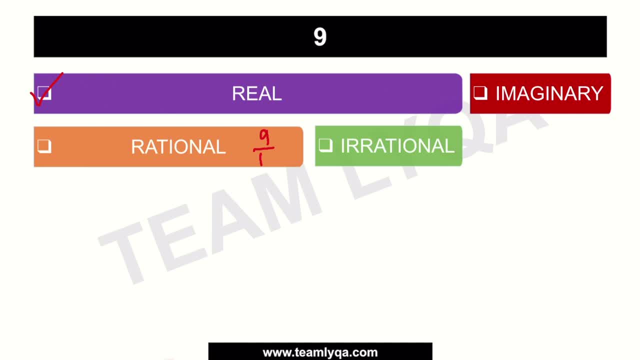 At dahil ang nine ay nine over one, at ang one ay hindi zero or yung kanyang nasa ilalim or denominator ay hindi zero, ibig sabihin siya ay rational number. Now, kung rational number siya, meron pa tayong susunod na level. 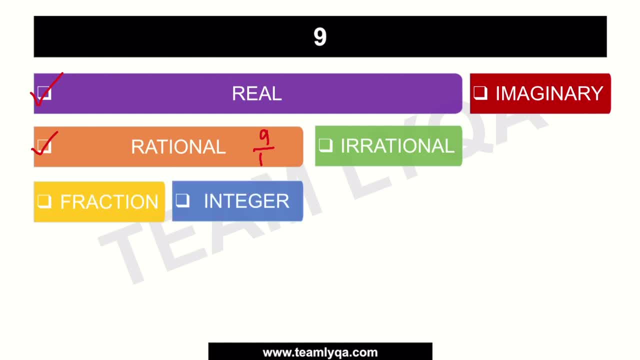 which is the question kung siya ay fraction o integer. Now, hindi siya fraction, sa pagkakasulat natin hindi naman required yung ating denominator. So ibig sabihin siya ay integer. 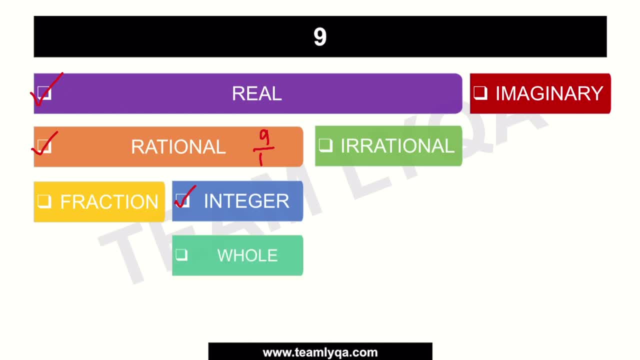 Now, kung integer siya, ang next question would be: whole number ba siya? Sabi natin, ang whole number ay lahat ng counting numbers at zero. So yes, pasok ang nine dun At natural number ba siya? 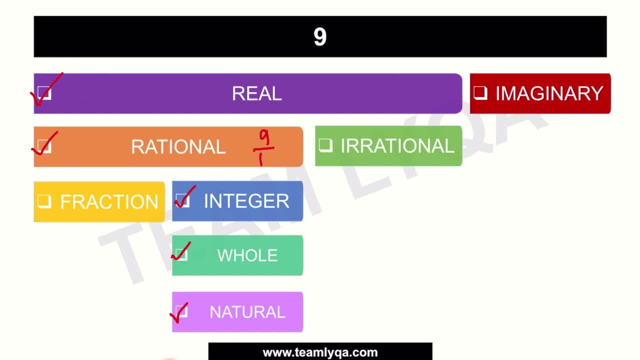 Yes, So check din tayo dyan. So ibig sabihin nun ang nine ay real, rational, integer, whole at natural. Okay, Now you can also look at this as a type of flowchart. 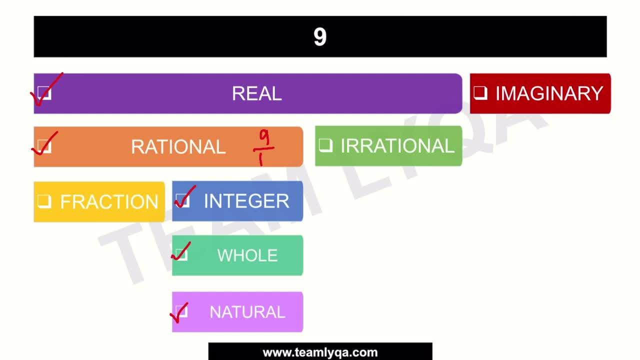 As you can see, a number can either be real or imaginary. Tapos, kung siya ay real, it can either be rational or irrational. Kung siya ay rational, it can either be a fraction or an integer At. kung integer siya, pwede siyang whole o hindi. 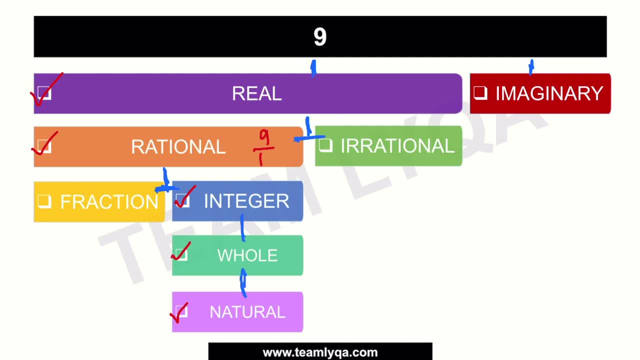 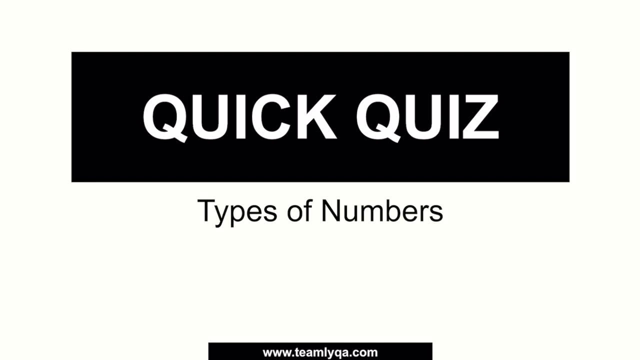 Kung whole siya, pwede siyang natural o hindi? Okay, So just something to think about Now. the best way for us to test if naiintindihan niyo siya is through a quick quiz. So if you're ready with your pen and paper, your timer starts now. 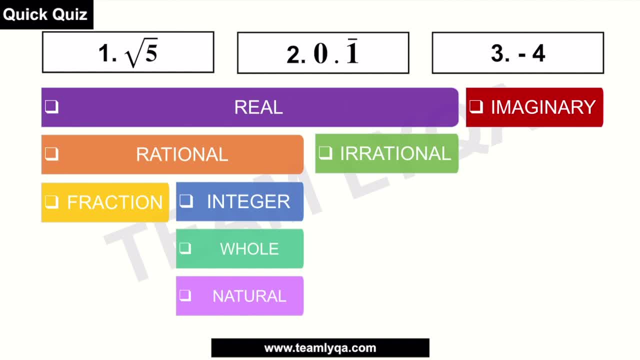 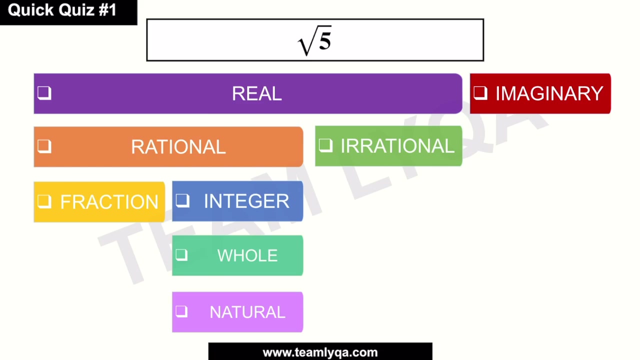 Let's begin. Alright, let's see how you did, see how you did all right. so let's start with the first one. it's the square root of five. now, first level, muna tayo real ba sya o imaginary. now dahil sya ay square root ng integer na hindi. 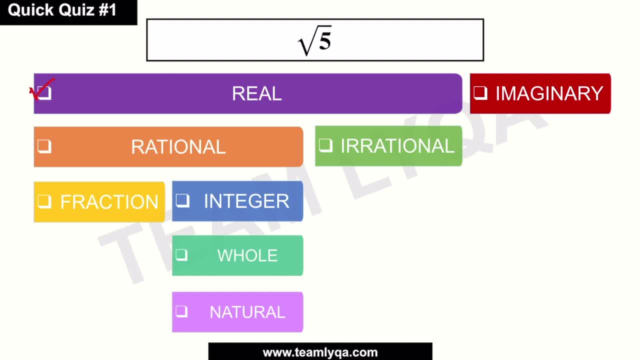 negative, ibig sabihin sya ay real, which leads us to the next question: sya ba ay rational o irrational? now you can use a calculator to find out kung anong square root of five or isa pa sa mga telltale signs ng irrational numbers ay yung mga square root na hindi perfect. 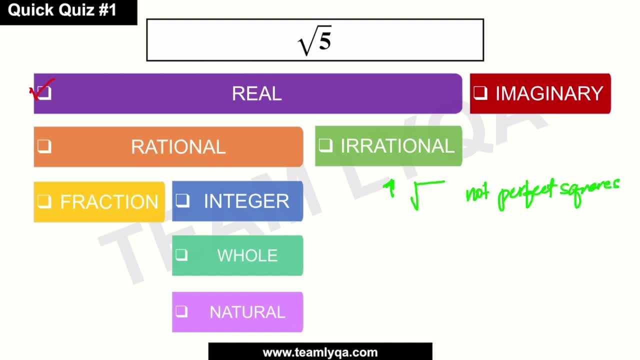 square, okay, square root ng number na hindi perfect square. now, hindi kasama doon ang square root of four, kasi yan ay two, pero ang square root of five, dahil hindi sya perfect square. it is actually an irrational number. at kung isosolve mo sya ang lalabas ay two point two, three, six, oh six. 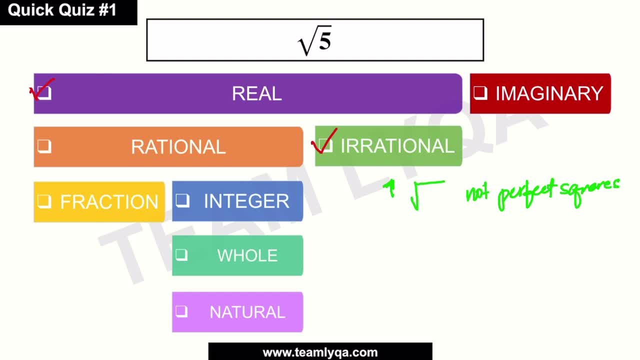 seven, nine, seven, seven, four, nine, nine, seven, nine at. hindi pa tayo natatapos doon. okay, now, dahil sya ay irrational number, hindi na sya pasok sa kahit ano dito sa left side na yan. that is all. there is square root. 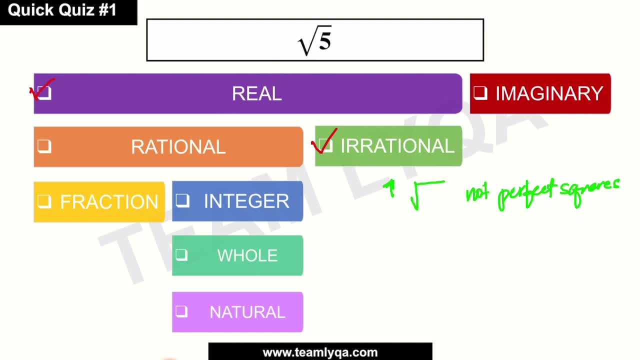 of five is a real number and also an irrational number. so number two naman tayo. you have zero point one as a repeating decimal. so zero point one, one, one, one, one, yan, yan, tuloy, tuloy tanong muna: is it real or imaginary? now, square root ba sya ng negative number, hindi, so ibig sabihin sya. 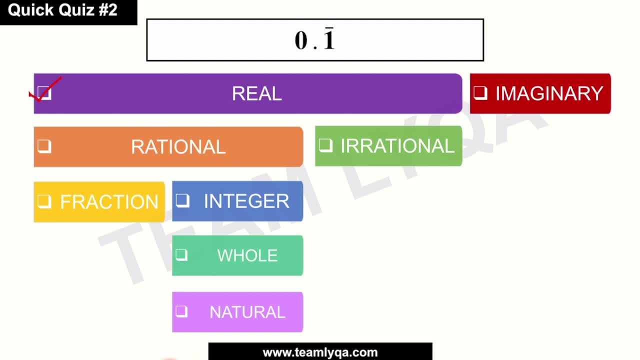 a real number, which leads us to the next question: rational ba sya o irrational? now, ang zero point one: kung isusulat natin as a fraction, yan ay one over nine. so ibig sabihin nun, dahil ito ay may numerator na one, denominator na nine, at ang kanyang denominator ay integer din at hindi zero. 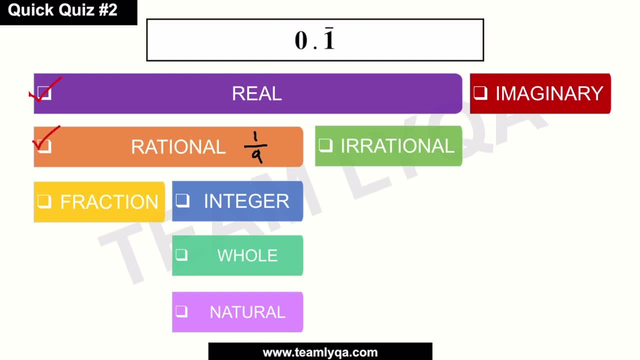 ito ay rational number. now, fraction ba sya? yes, no one thing we have to understand is that decimals can also be written as fractions. wala syang kung. wala syang decimal kung whole number sya. we would go through the entire list here. pero dahil fraction na sya, tapos na tayo dyan. 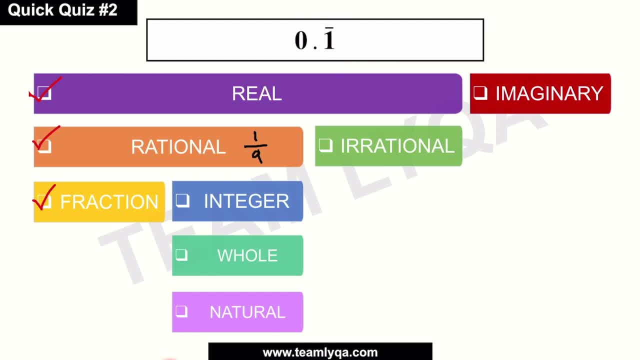 zero, point one, na repeating decimal ay real, rational at fraction. doon tayo sa number three. you have negative four, which is a real number. no, hindi sya imaginary, hindi sya square root of a negative number. now, rational ba sya o irrational? ang negative four ay pwede mong isulat as negative four over. 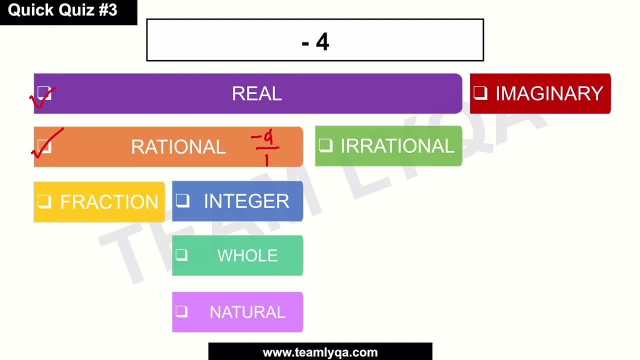 one. so ibig sabihin nun rational din sya. now, buo naman syang number. no, hindi required na isulat sya lagi sa fraction form. so ibig sabihin nun integer sya. pero ang question would be whole number ba sya? now dahil ito ay negative? no, dahil negative sya, hindi na sya. whole, hindi na sya. 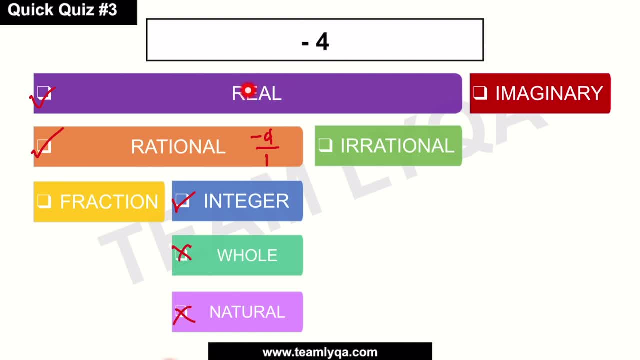 natural. so negative four is real, rational and an integer okay. now i hope yung ating table, yung ating mga diagram helps you master this. kasi again bonus points sya pagdating sa mga college entrance test or science high school test, sana no, kung 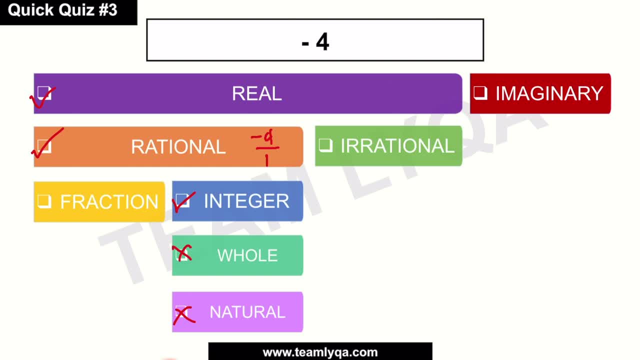 makukuha nyo sya agad and i hope na padali kahit papaano yung pag determine nyo kung alin ang alin. all right. if you want more exercises, i'll be posting more questions on my instagram account. 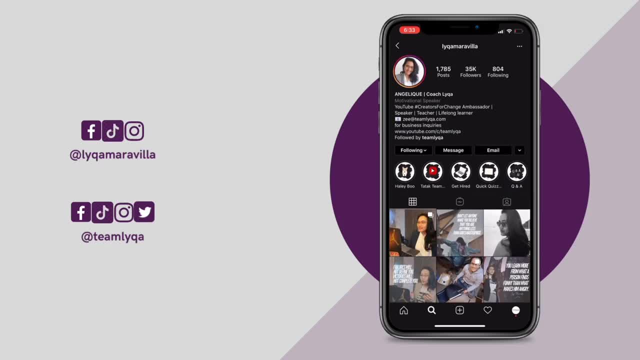 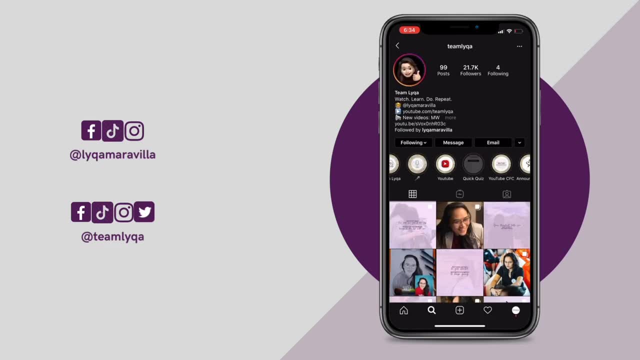 so if you don't follow me yet on instagram, you can follow me at like a maravilla on instagram for the new quick quiz questions na pinapost natin sa ating instagram stories. and if you want the throwback quiz, quick quiz questions, naman nandun sya sa at team laika on. 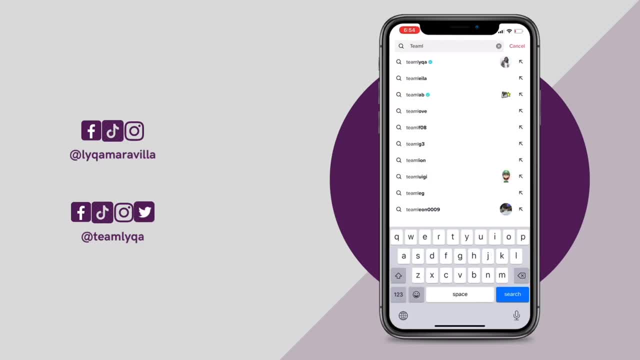 instagram. you can also check out my tiktok accounts at team laika for the educational videos- math, science, logic, at iba pa and at like a maravilla naman for the more personal stuff, yung mga vlogs, motivational videos, tips and advice. all right, i'll see you online. all right, i hope you learned. 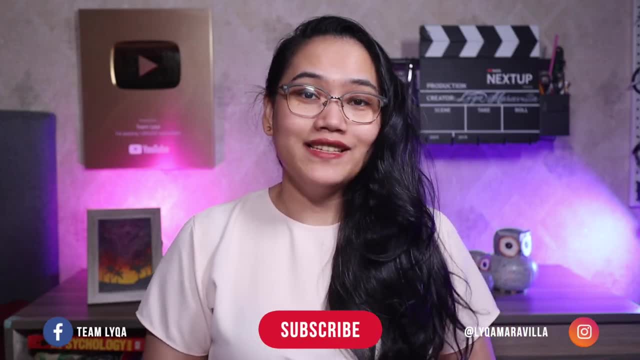 something today. if you did click thumbs up, make sure that you share this video with your friends. natin masalami, tayong matutulungan. and, as always, if you want to reach out to me directly, get the reviewers that i made, join the online or live chat and i'll see you next time. bye, bye. 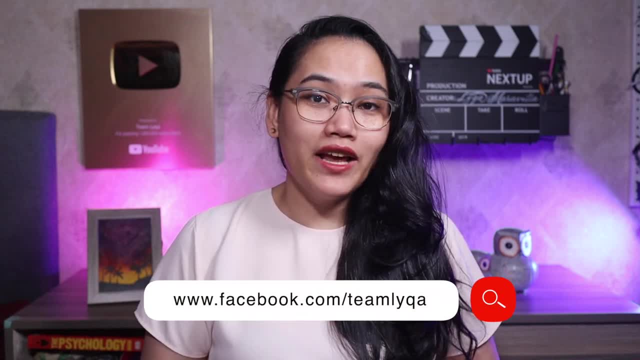 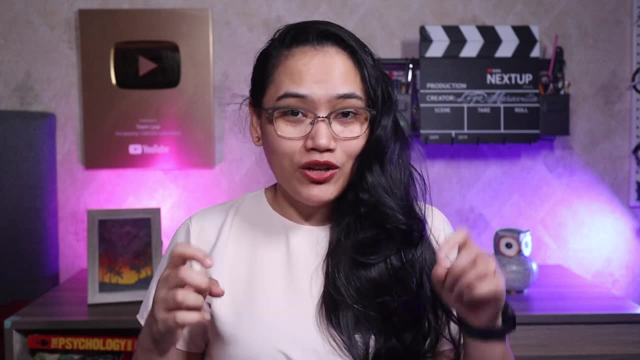 review events. you can go to the wwwfacebookcom slash team laika for more information. all right, don't forget to subscribe. hit that bell icon. we have more videos coming up and kung meron din kayo request na topic, pwede nyo i-comment sa baba, i'll see you on my next video, never stop. 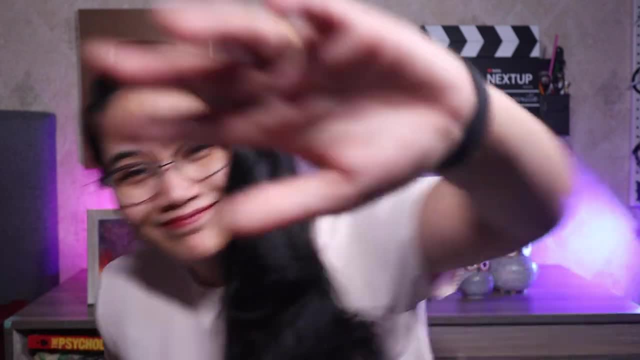 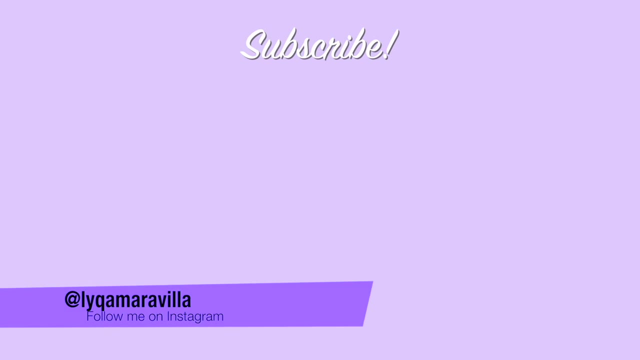 learning. adja adja kain yan bye for now, you.